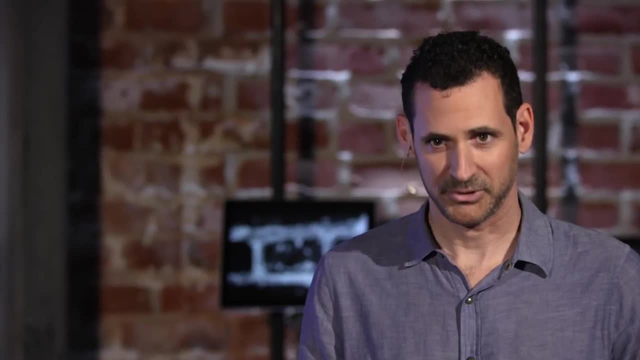 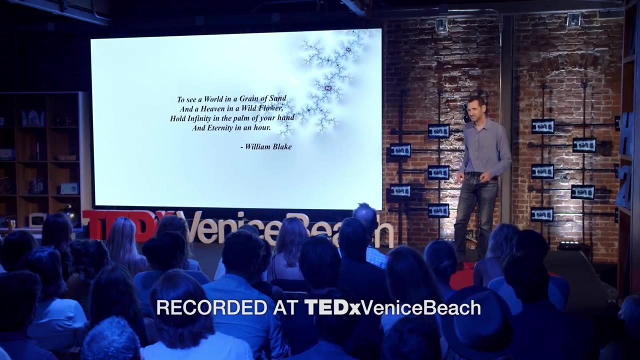 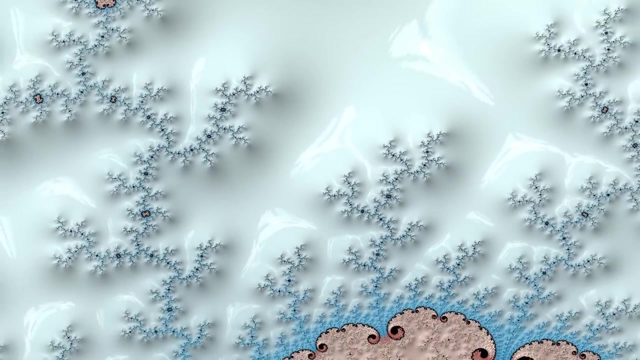 but I think we can all agree that this poem is about fractals, and that's pretty impressive because because fractals weren't discovered until a hundred and seventy years later. but Blake's poem captures something essential about the natural world around us. It draws a connection between the very large and the very small. 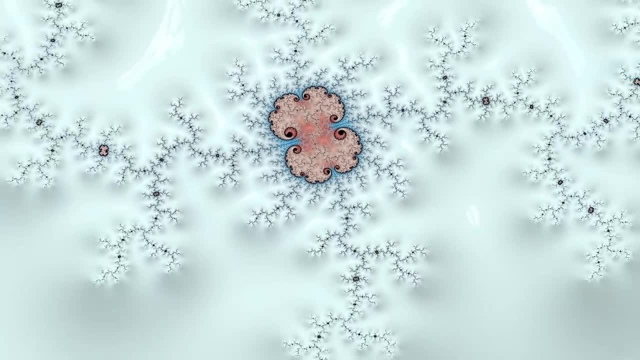 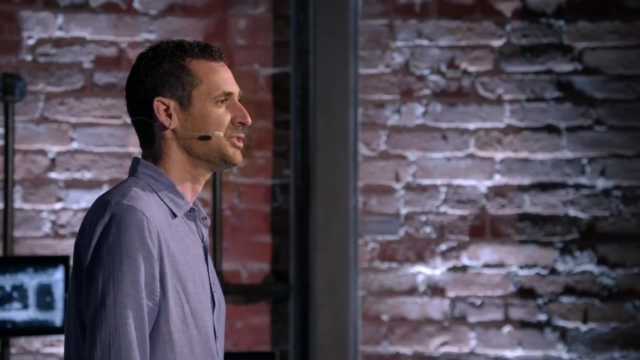 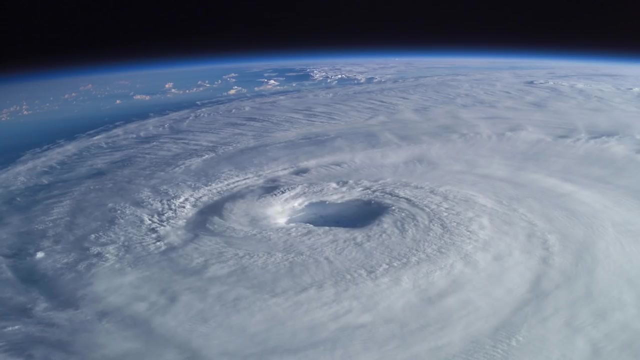 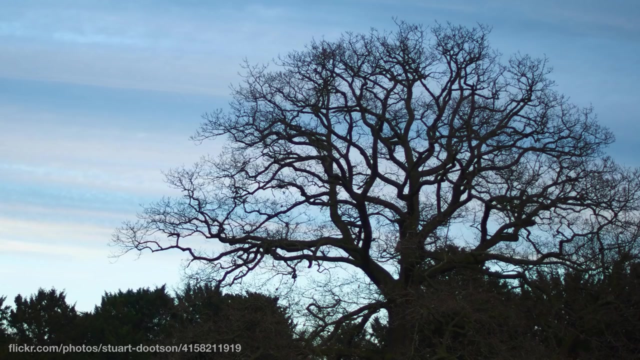 and it observes that similar patterns can occur at vastly different scales across time and space. and we see this in the universe around us: Similar patterns from the shape of immense spiral galaxies to the weather patterns of a hurricane, to little eddies in a stream, and whenever you have a single object that contains these patterns, repeating. 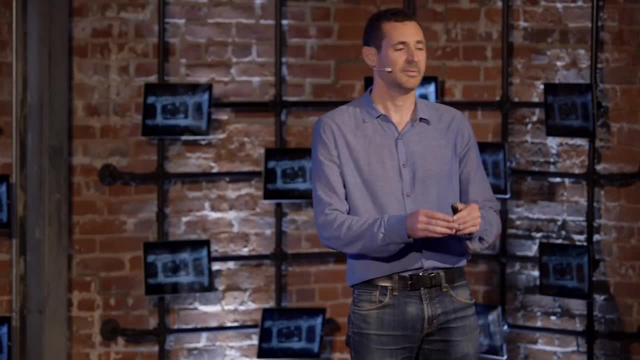 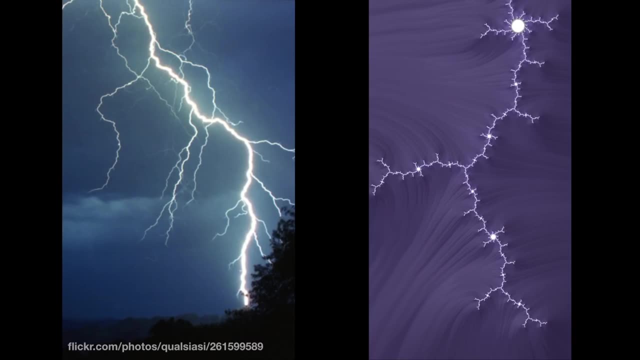 over and over again, at many different scales and where every small part resembles the whole. that's a fractal, And we see them around us everywhere, from the jagged shapes of lightning bolts to the rough, ragged edges of coastlines. 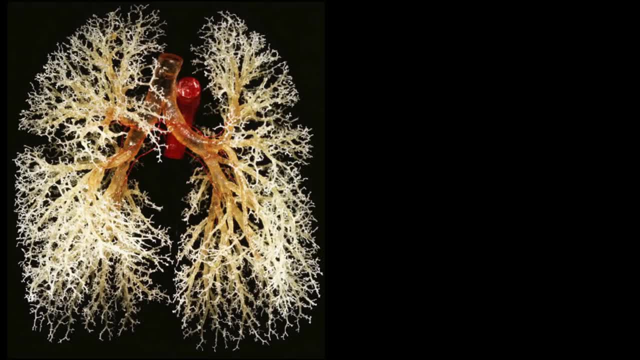 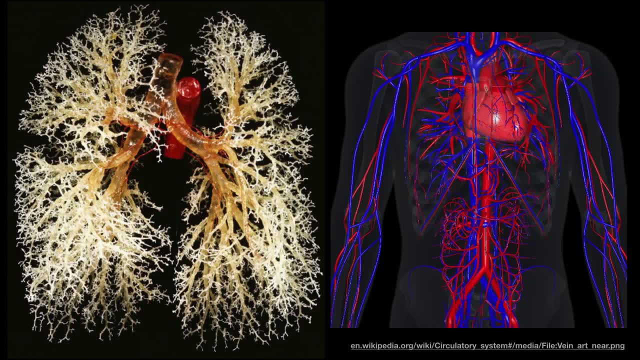 But fractals are not just outside of us. Our lungs are fractals. That's how they manage to pack the surface area of a tennis court. fold it down into your rib cage And our circulatory system is a fractal as well. 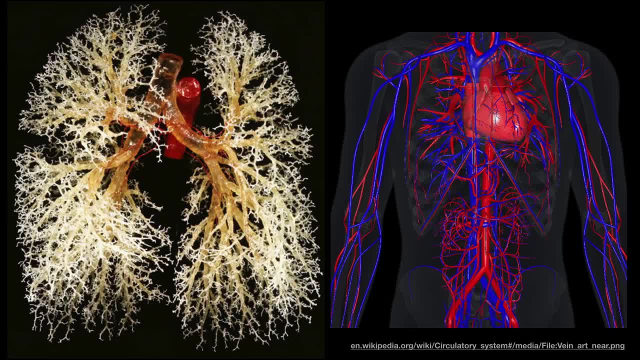 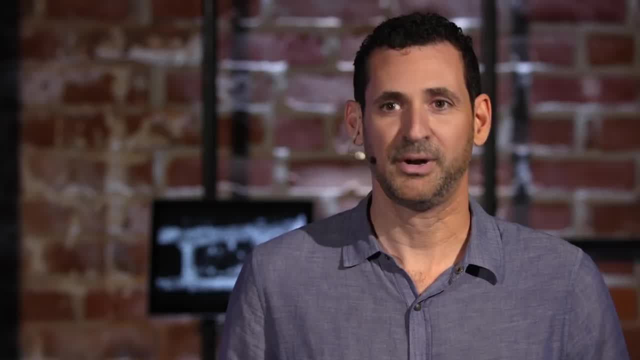 which is how 60,000 miles of branching blood vessels and capillaries fit inside every human being. So I'm able to stand here and talk to you today because I'm the living breathing fractal, and so are you, But for hundreds of years. 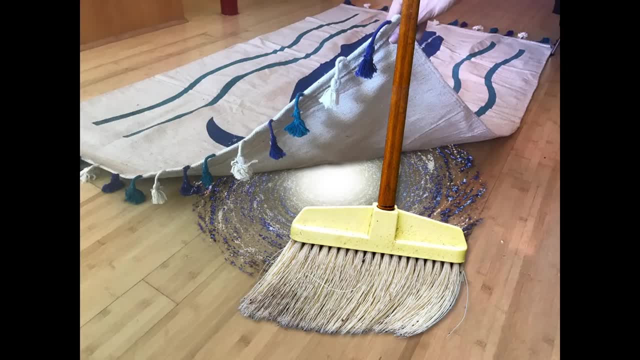 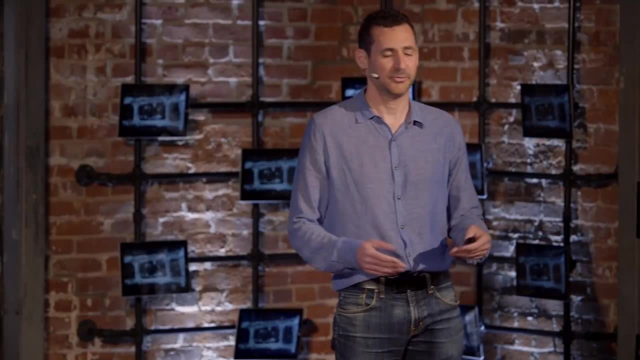 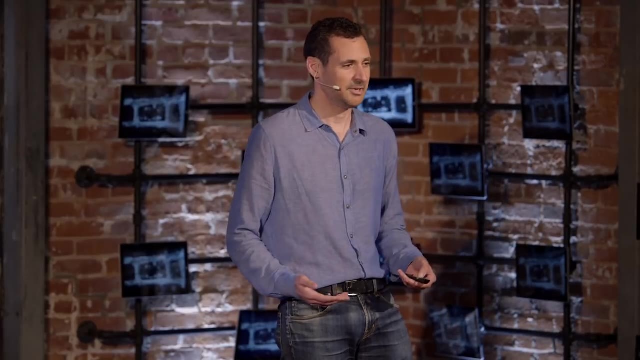 these complicated geometric shapes were swept under the rug. They were considered too complicated to mathematically analyze because they don't behave like circles or squares or triangles, And the assumption was that any explanation for these shapes would have to be as complicated as the shapes themselves. 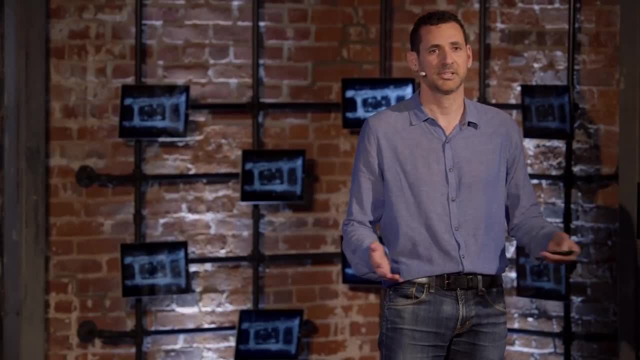 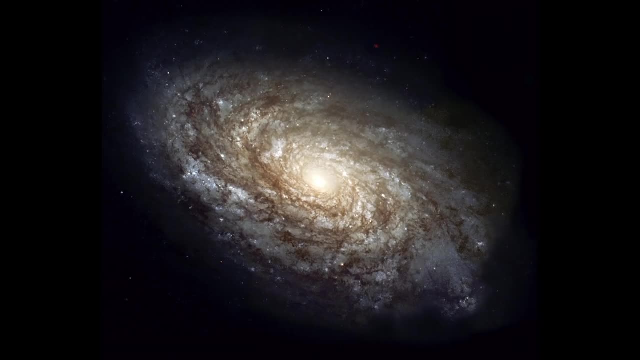 Because ordinarily simple things have simple explanations and complex things have complex explanations. But every once in a while something comes along that breaks the mold. Take the universe. A hundred years ago there was a crisis in physics Measurements of the natural world. 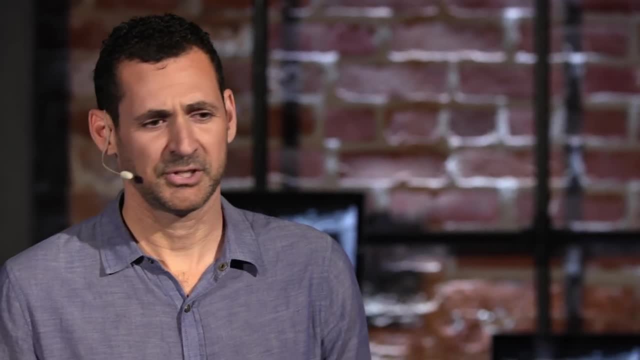 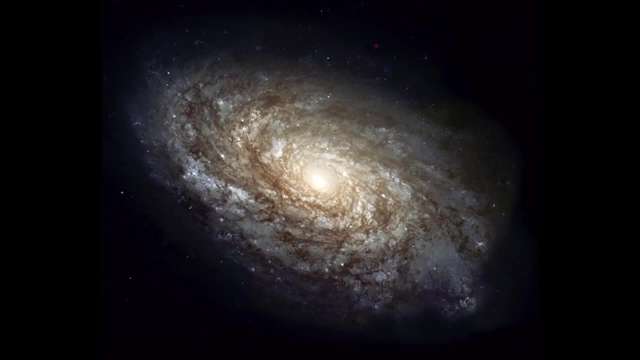 weren't working out the way that scientists expected, And physicists were tying themselves in knots, coming up with more and more convoluted theories trying to explain away these discrepancies. But then this guy showed up with a very simple equation, And this led to the discovery of the theory of relativity. 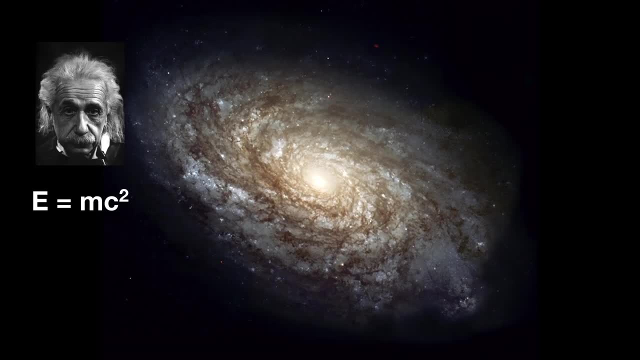 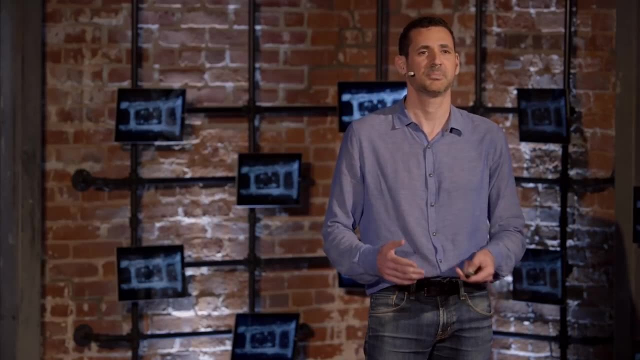 that opened up an entire new era in physics. Seventy years later, geometry was in a similar crisis, because mathematicians still couldn't explain the properties of these complex shapes. But then this mathematician, Benoit Mandelbrot, found himself studying an equally simple equation. 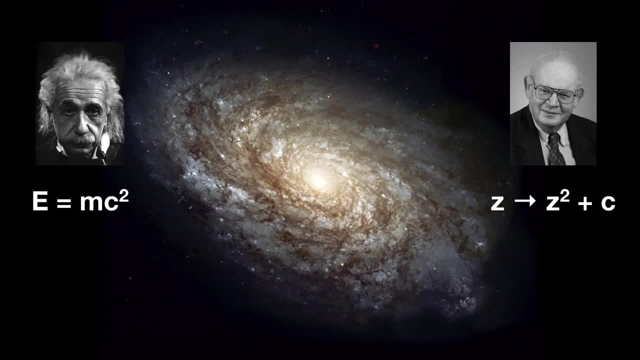 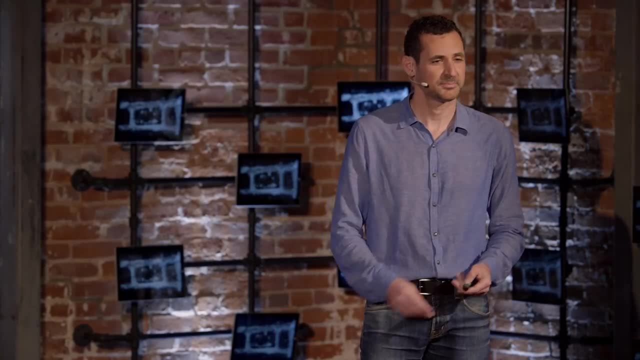 And from this simple equation. this unlocked the mysteries of these complex shapes And it led to the development of the entire new fields of chaos theory and fractal geometry. So let's take a look at this equation: Z goes to Z squared plus C. 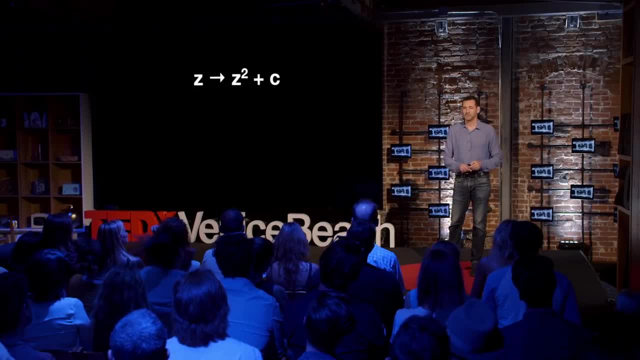 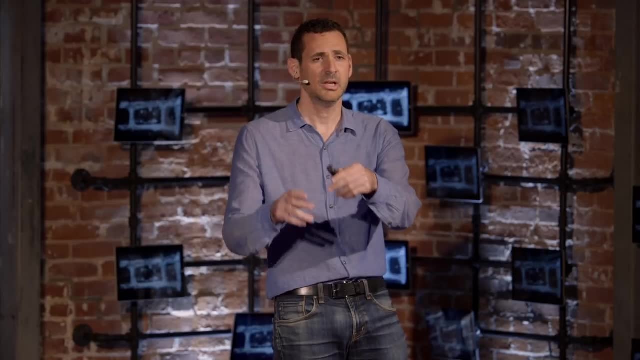 And the way that this works is that you take a small number, you square it, you add the original number, then you feed that back into the equation square, it add the original number and you process it over and over each time, feeding back in the original number. 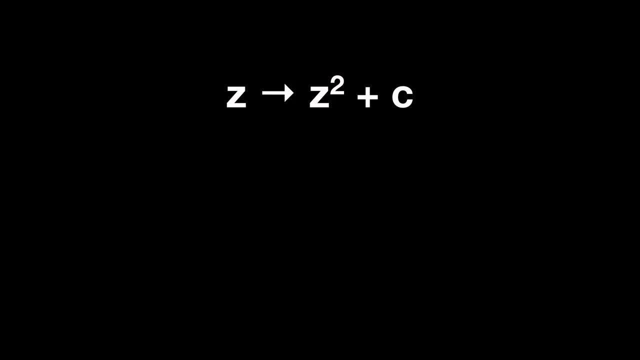 to keep the process going. And for some numbers not much happens, It just stays small. For other numbers it just bounces back and forth. But for other values it grows very quickly and it quickly escapes to infinity, And it's possible to compute this by hand. 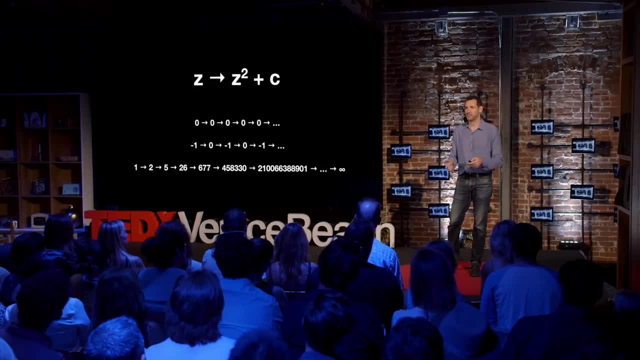 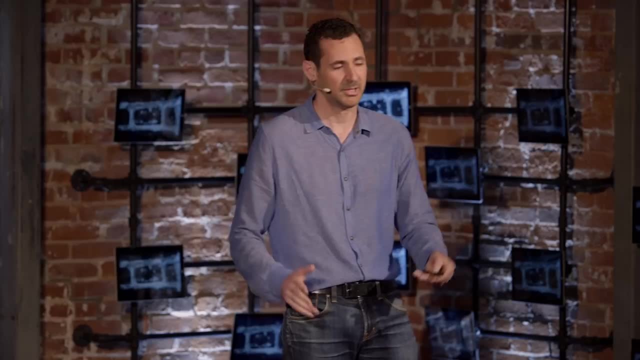 for 10 or 100 or 1,000 different numbers. But to get a true idea of what's really going on you need to do this with a computer for millions and millions of numbers in two dimensions. And when you do that and plot the results, 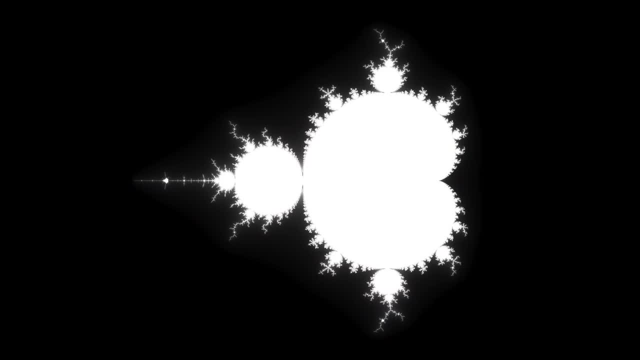 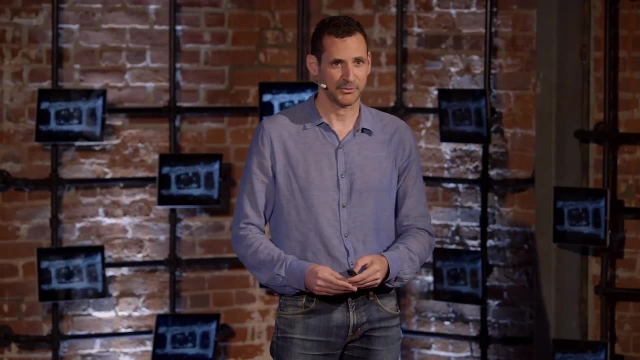 you get this fantastic shape. the Mandelbrot set a shape of infinite complexity generated from such an incredibly simple formula. This shape changed my life. Now, my parents' first inkling that I was mathematically inclined was when I was quite small. 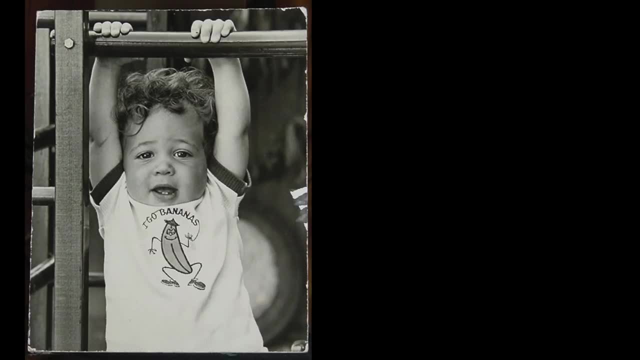 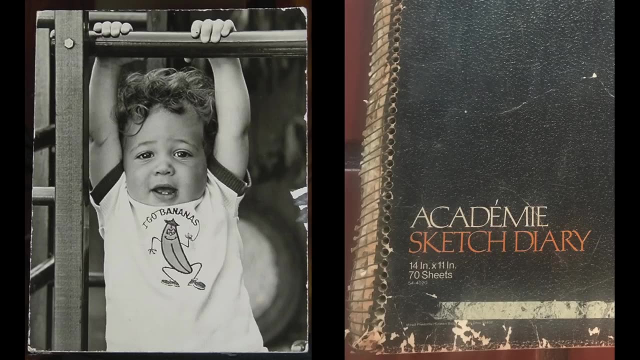 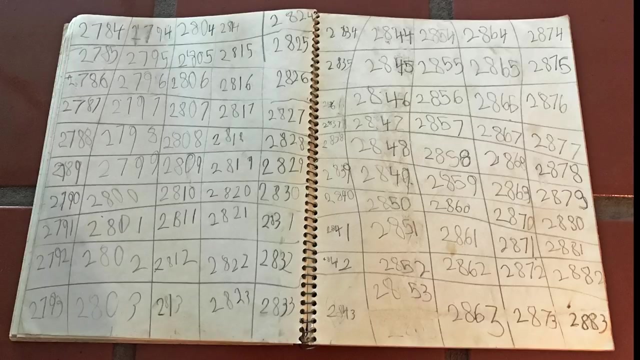 and I announced to them that I was going to count to infinity, And so they humored me and they bought me a 70-page notebook And I got started And it was going along pretty well. I think I was actually getting most of the way there. 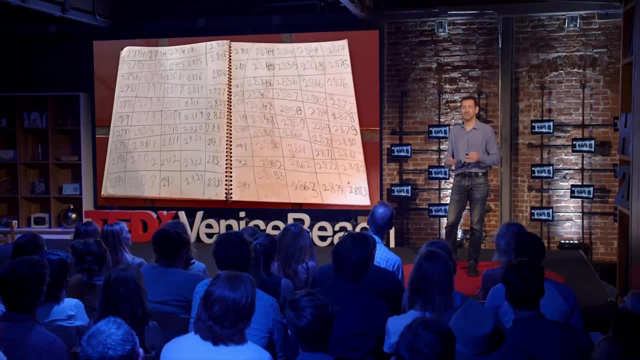 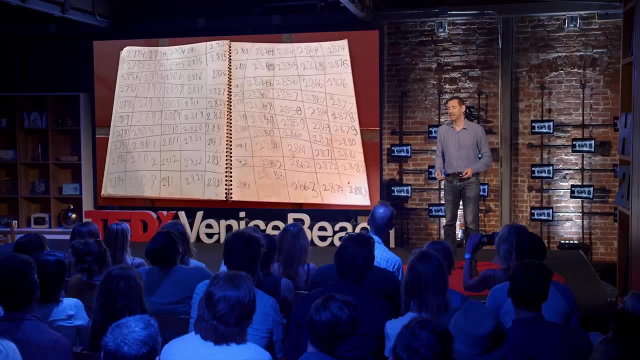 And so, as you can imagine, when I discovered that I could make a computer do this sort of thing for me and also produce images as complicated and as amazing as the Mandelbrot set, I was completely hooked. I would write a computer program. 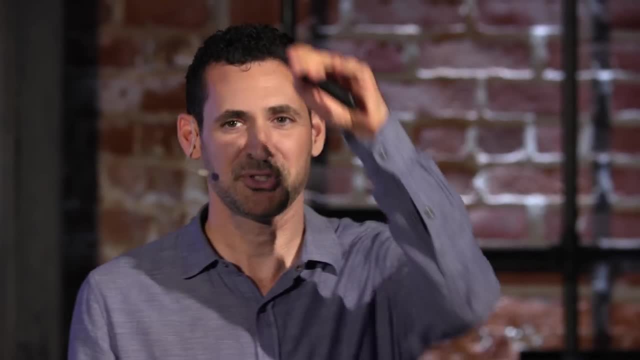 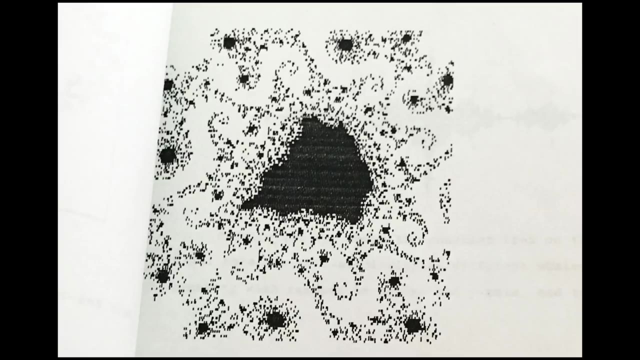 go off to summer camp for a week and run back to find that it had almost finished drawing one picture of a fractal. This image was from a paper I wrote in the ninth grade and it literally took the computer a week to draw. 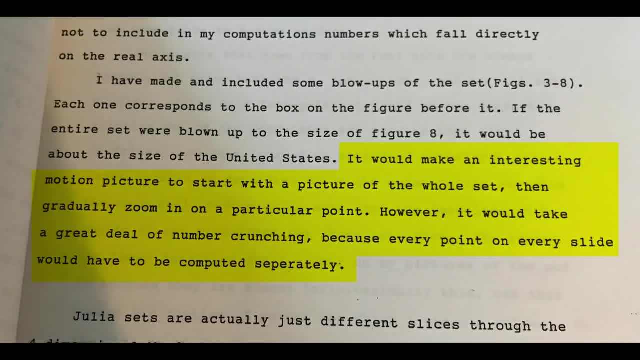 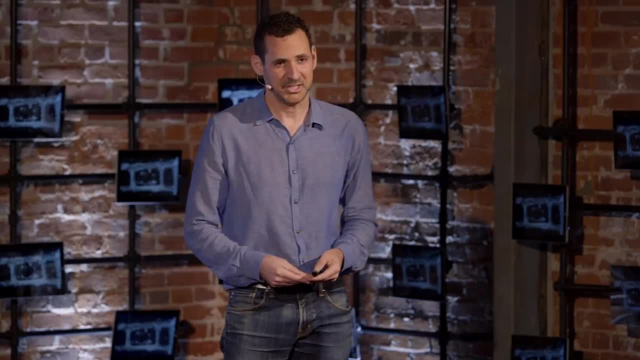 But in that paper I had this crazy idea: I thought that if you could make enough of these pictures and put them back to back, you could make a movie of flying through the Mandelbrot set, Of course, in the 1980s. 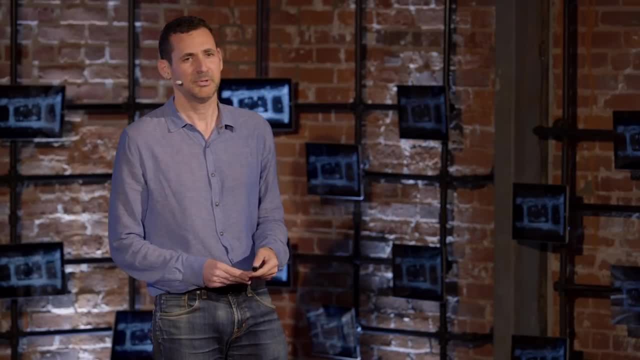 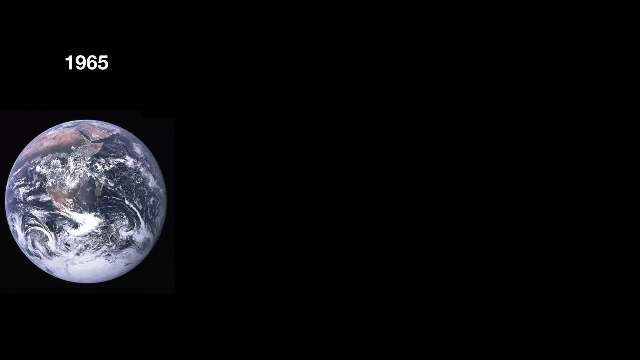 that was a crazy pipe dream on a home computer, But fortunately computers have gotten a little faster since then. For perspective: in the Apollo era in the 1960s the sum total of all the computing power in the world was about 10 gigaflops. 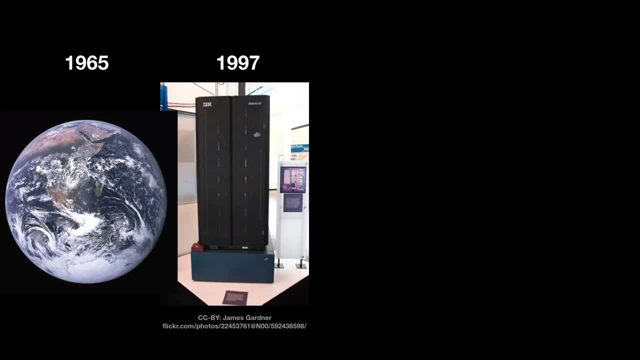 about 10 billion instructions per second. By the late 90s, IBM was able to pack all of that power into a single supercomputer the size of a refrigerator. By 2011,, it could fit into your pocket And, extrapolating ahead just a few years, 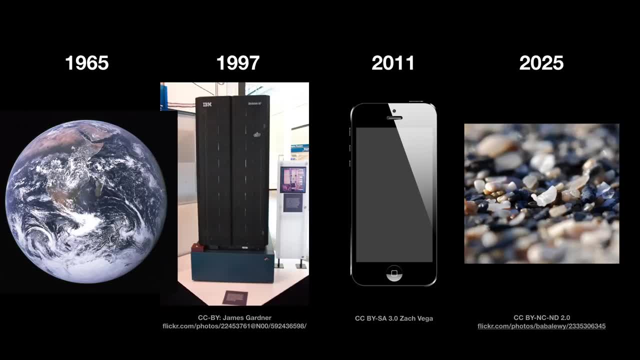 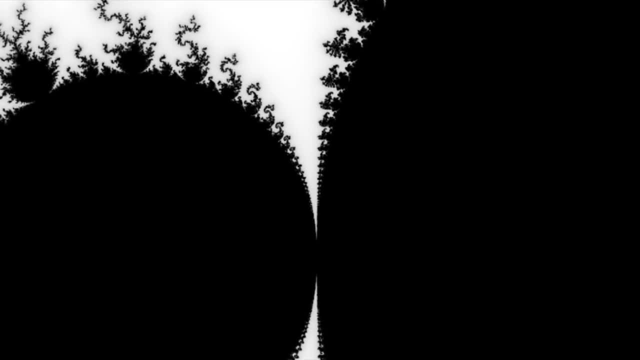 all that power will be able to fit into a single grain of sand. So let's do that: zoom into the Mandelbrot set. And now it can be done in real time on a cell phone, And so I'll zoom in just a little bit. 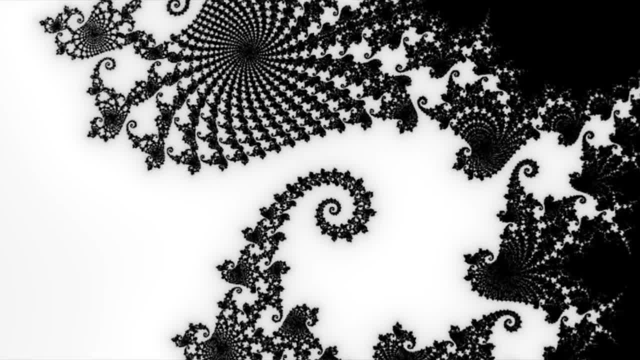 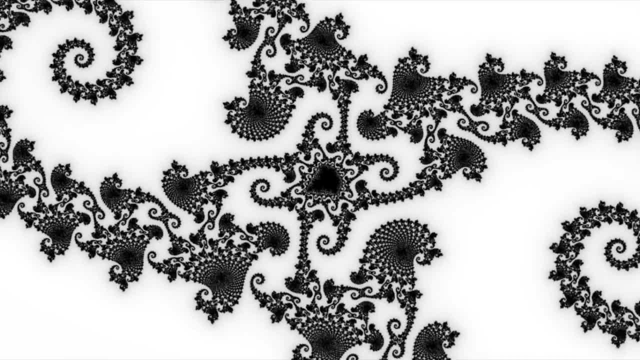 And by a little bit I mean a factor of 100 million, because mathematically there's no reason to stop there. This shape literally goes on forever. You really can hold infinity in the palm of your hand. And in addition to all of the geometric complexity, 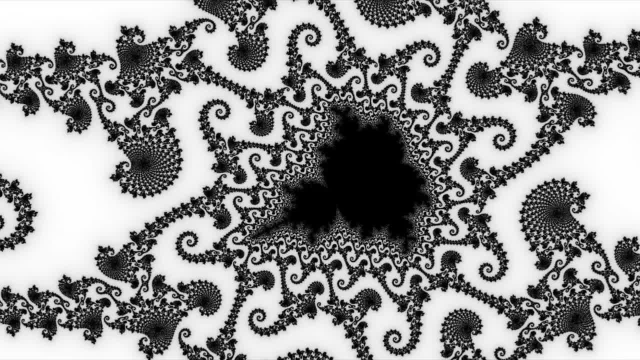 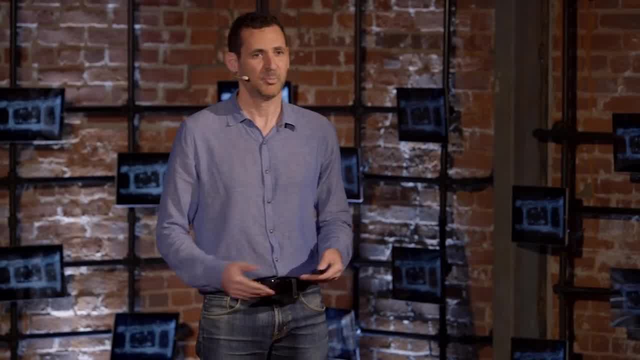 you can see the self-similarity that buried deep down within the Mandelbrot set are little copies of the original shape. In 2010,, Mandelbrot himself gave a talk at the TED conference in Long Beach, And I was lucky enough to be there and to get to meet him. 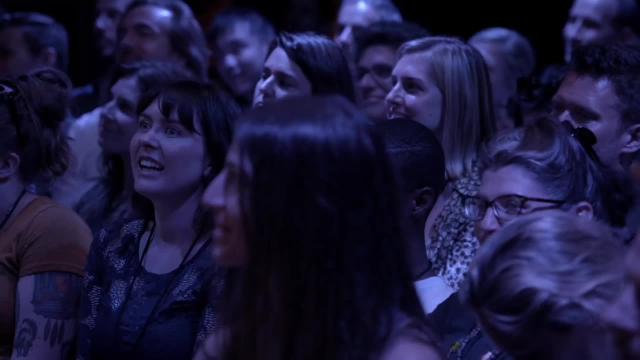 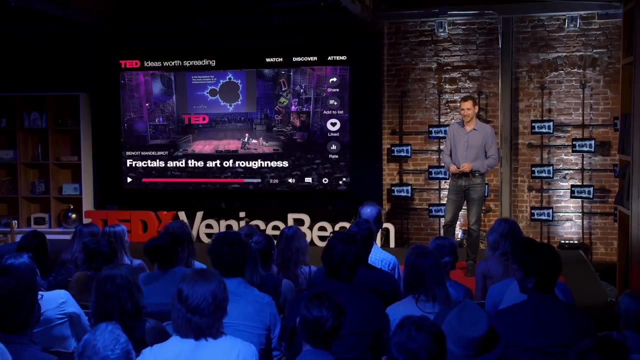 And, as you can imagine, that was a real TED moment for me And I think he would have appreciated that buried deep down within my fractal talk is a little copy of his fractal talk, And so I showed him what I was working on. 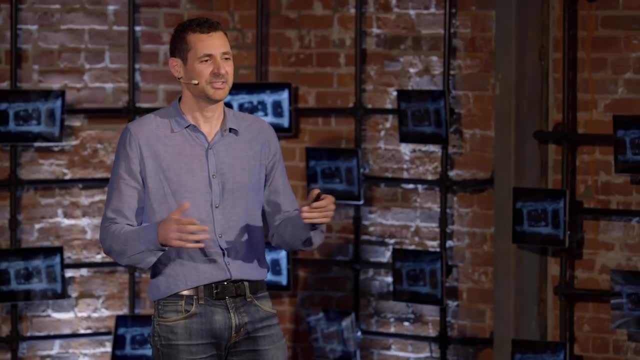 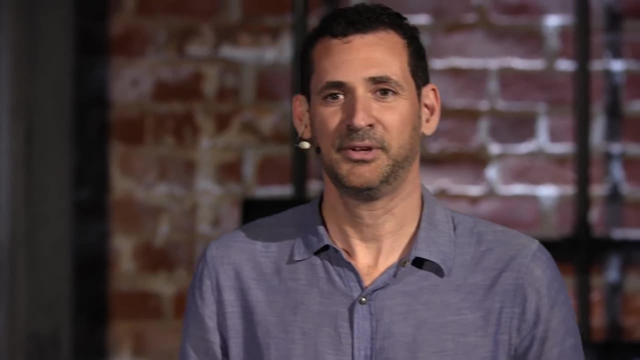 this program on the cell phone to fly into the Mandelbrot set And he was amazed. He said it was superb that such a thing could now be done on such a small device And it felt like the passing of a torch And I felt like I should run with that. 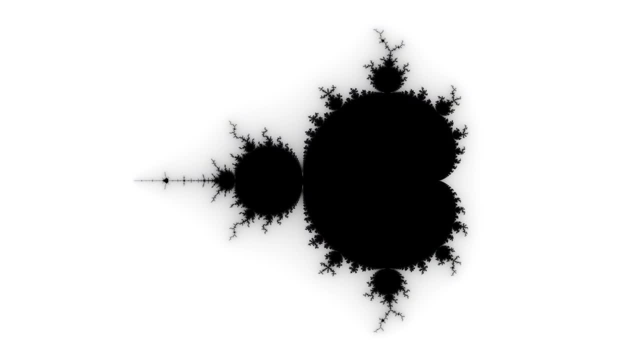 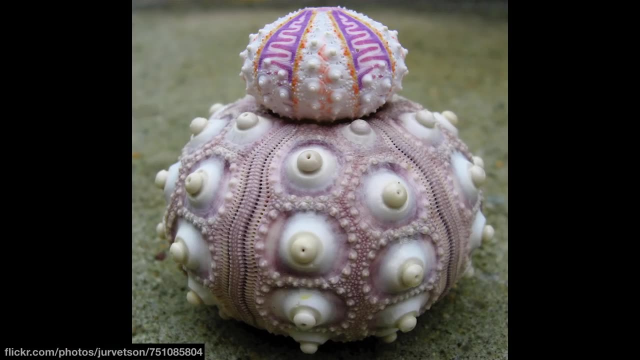 And I wanted to run with that as far as I could. Now. the Mandelbrot set is very beautiful all by itself, But when you look at natural fractal shapes that occur in the real world, they have color and shading and lighting and texture. 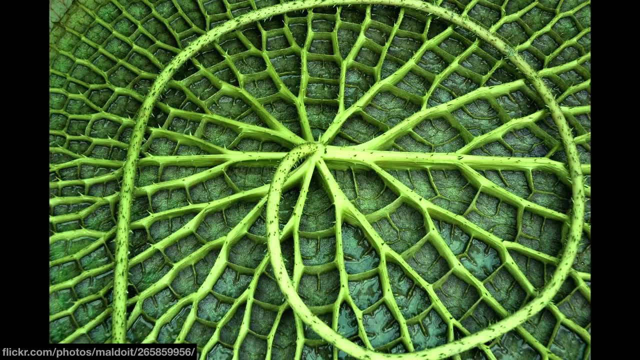 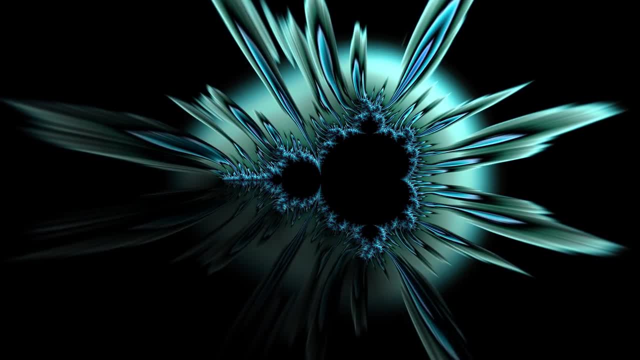 And I wanted to bring that into the images that I was creating. And I found that if I took the space surrounding the Mandelbrot set and distorted it using techniques similar to that used for paper marbling, not only it would give it much more visual richness and complexity, 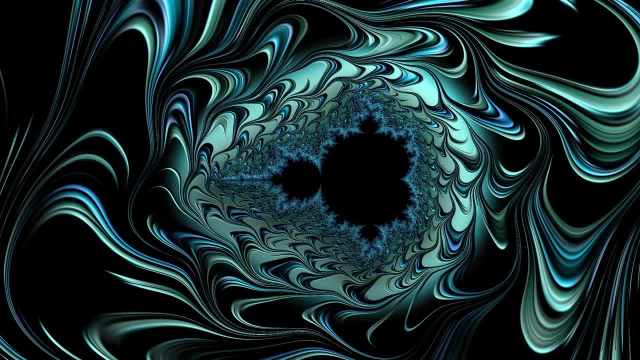 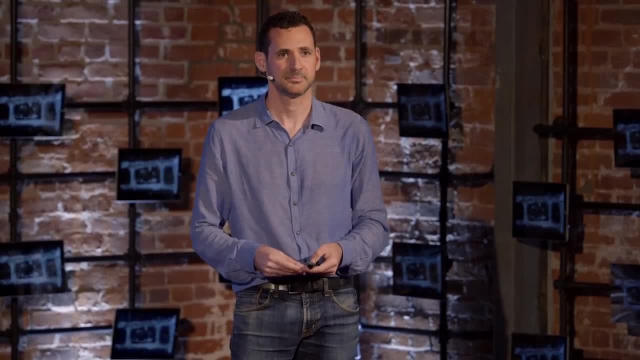 but it also reveals more of what's happening mathematically in the area outside the shape. Just as when you put smoke into a wind tunnel, it reveals patterns in the airflow that would otherwise be invisible, And so, using this technique, here are just a few of the textures and patterns. 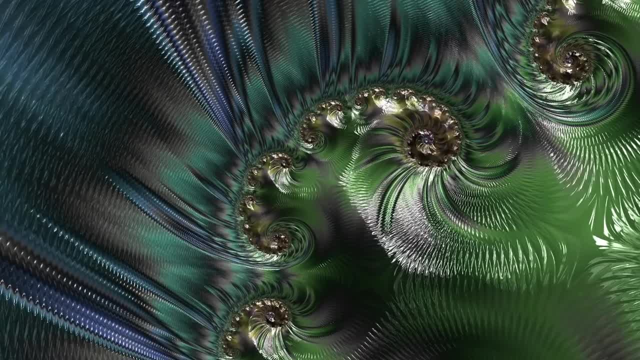 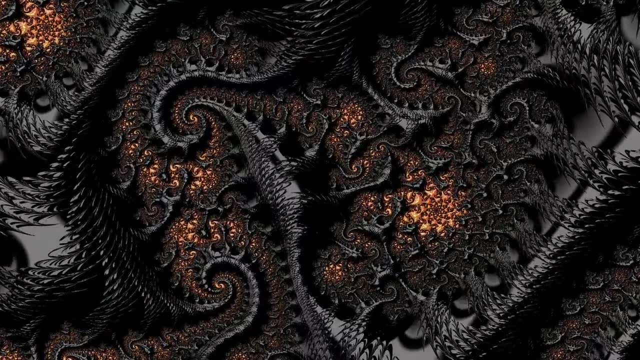 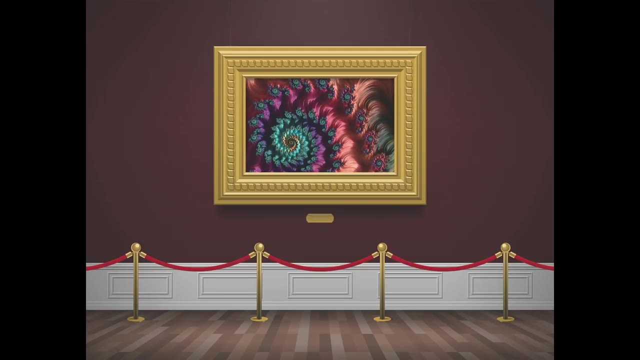 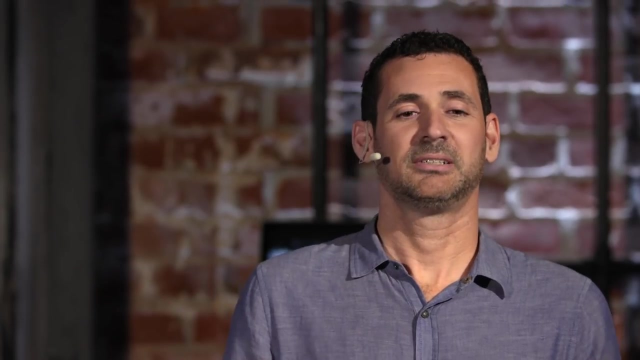 that we've uncovered hidden in the math. Occasionally, someone will tell me that these images belong in a museum. But I think that's a terrible idea, because at the museum the first thing they tell you is: don't touch the art. But we're all walking around now. 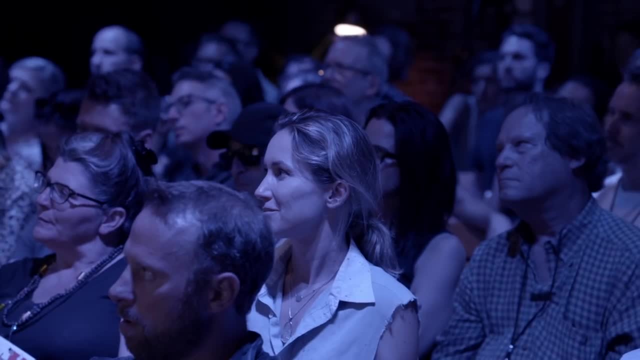 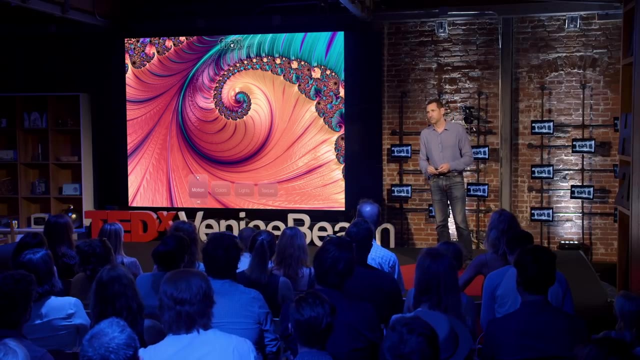 with touchscreen supercomputers in our pockets. Fractals should be all about touching the art. It should be an interactive, immersive experience, And so that's what I set out to create, working with a legendary graphic and user interface designer, Kai Krause. 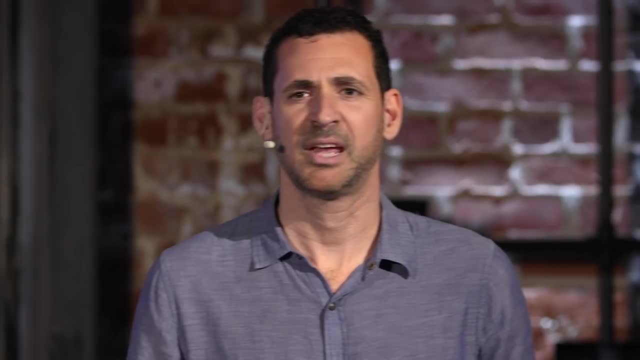 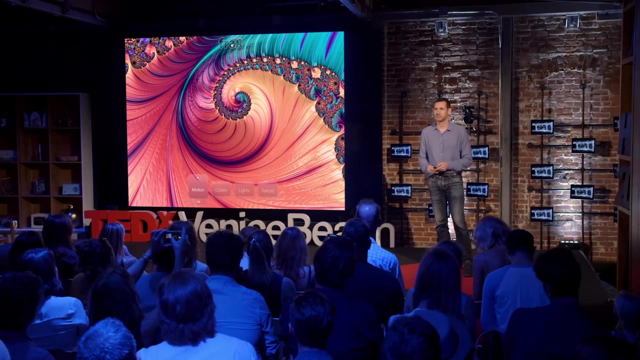 and another fractal expert, Tom Bedard. This is the app that we came up with, And you might notice that something is missing. There are no numbers or equations or scary math, And that's very intentional, because we do want to get people excited. 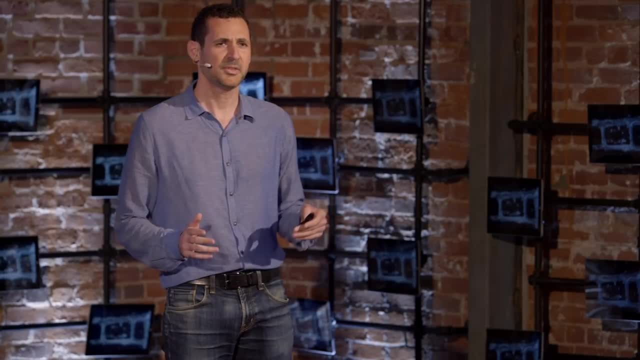 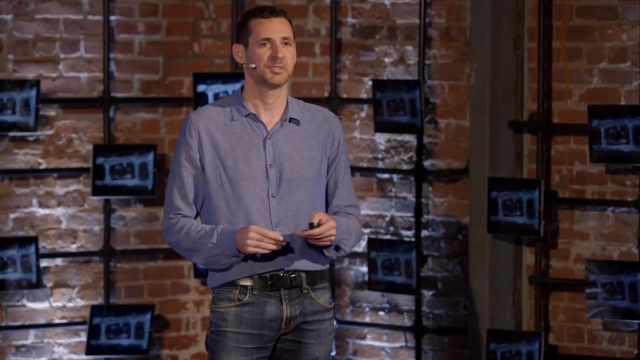 and interested about math, And we think that the best way to do that is not to shove a bunch of math in their faces, but to show them something inspirational and inspiring that can be done with math, and let them discover the inspiration all for themselves. 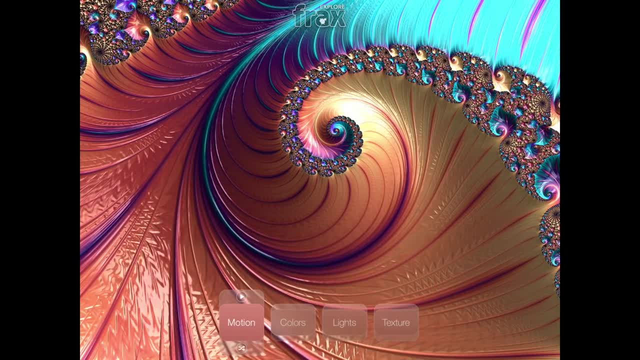 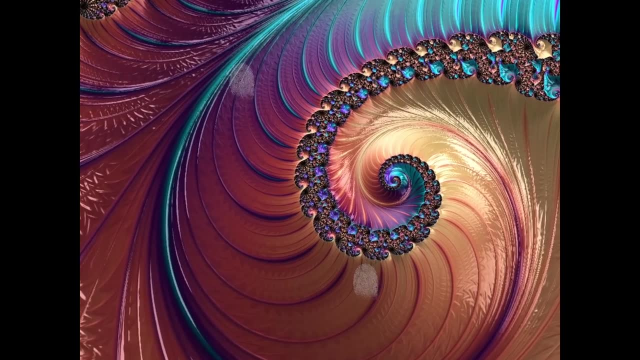 And so this is the app in action, And when you're actually interacting with these fractals, the interface completely goes away and you can just interact completely immersively. And even when you zoom into the fractal, you don't even need to touch to tell it where to go. 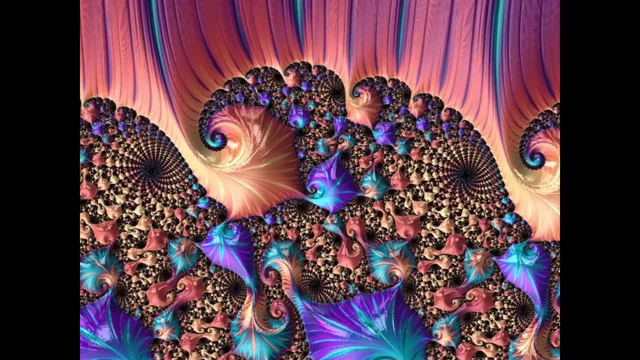 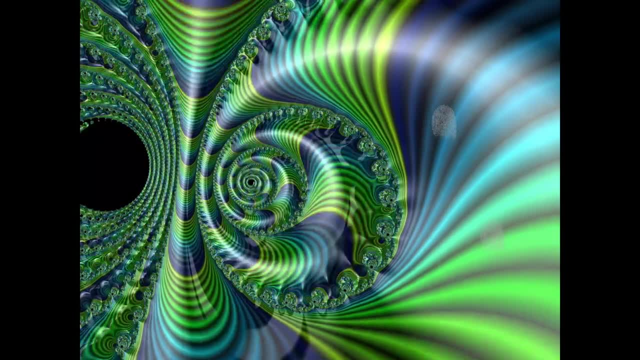 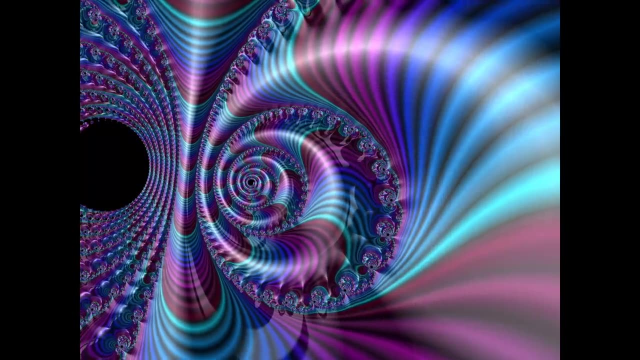 You can just tilt your phone to steer and it feels just like you're flying. And you can change the colors as well: pinching and stretching the color gradients around the fractal, swiping to animate them, rotating to change the colors and the hues. 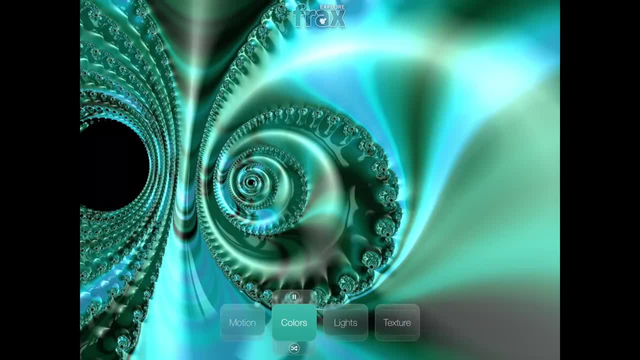 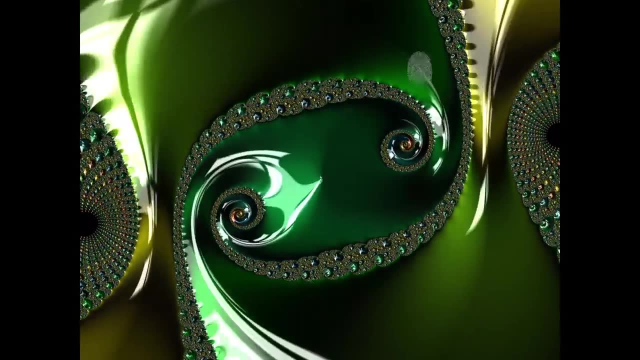 or randomizing your way through any number of different color palettes until you find one that you like, And you can change the lighting as well in a similar way. Move the lights around, swipe to animate them, pinch and stretch to make the fractal more or less depthy. 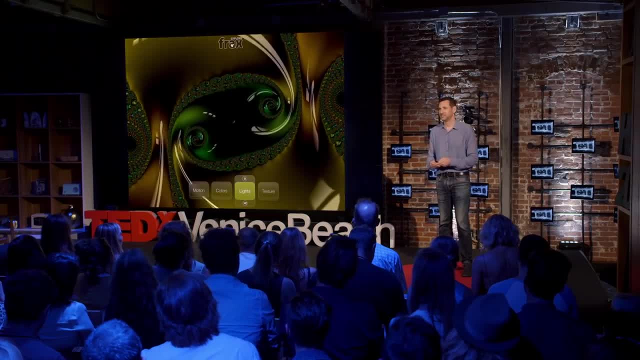 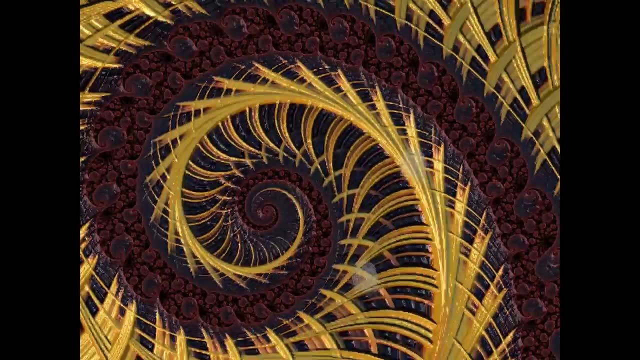 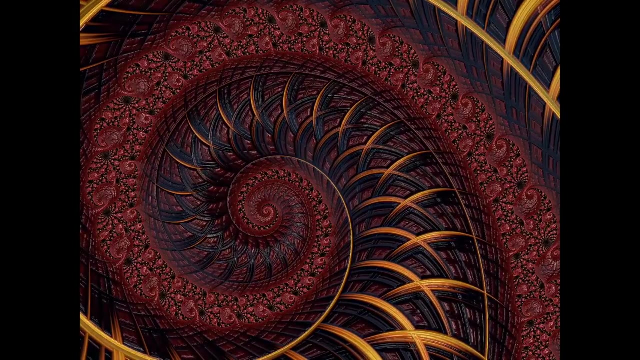 And my favorite is the texture, which you can interact with directly as well, changing the surface characteristics and properties, stretching and twisting it, and also randomizing through many different variations on a theme, And a whole community has built up around these tools. 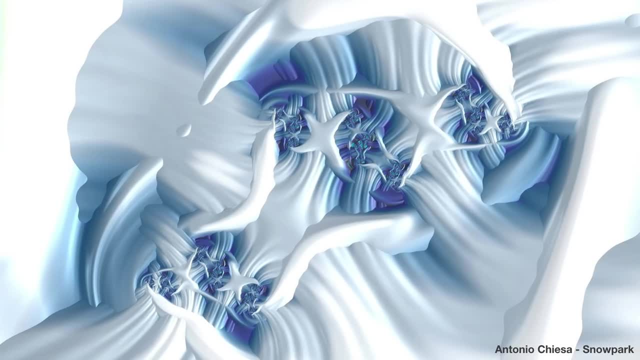 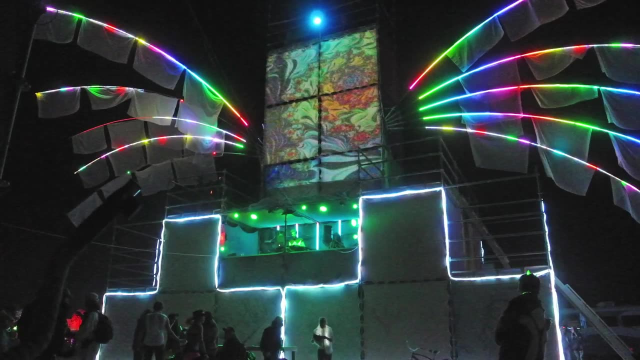 of artists from all over the world and we're consistently amazed by their artistry and creativity. But fractals also tend to draw a crowd. A few years ago I was invited out to Burning Man to show these fractals on a big video wall. 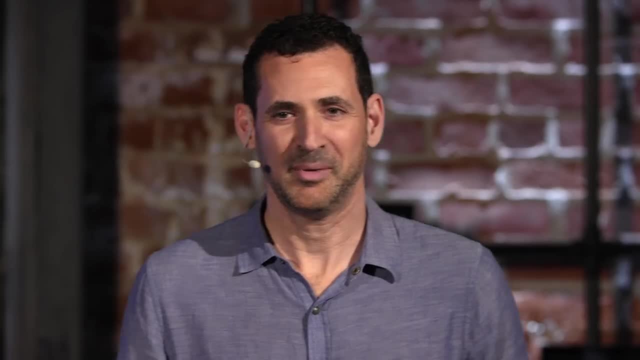 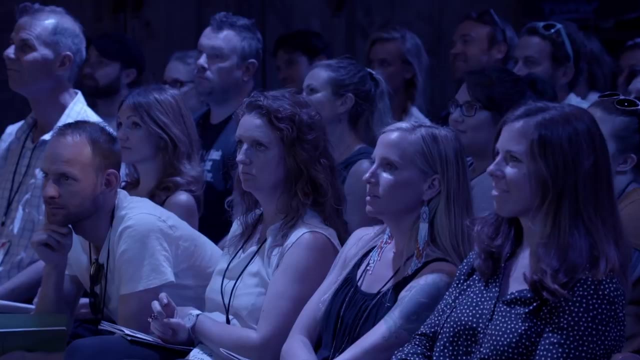 in the middle of the desert And people in the audience could come up and control and steer the fractals themselves from a tablet. And of course, being Burning Man, I had to make a costume, So of course this is an electroluminescent Mandelbrot. 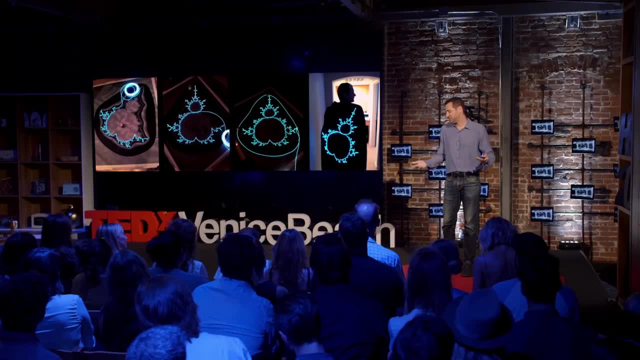 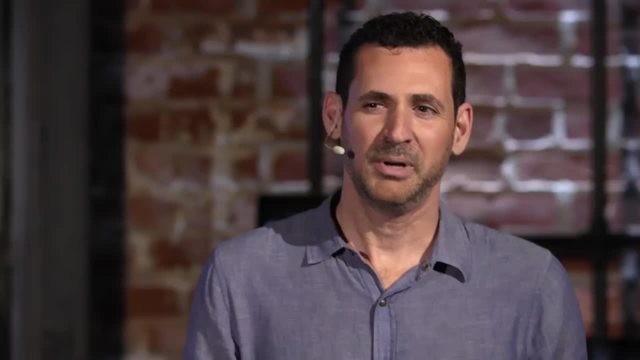 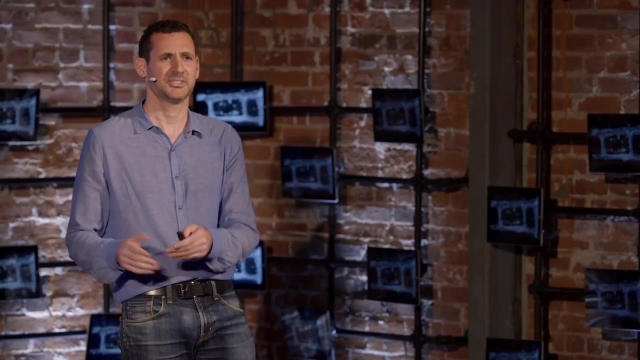 stitched onto the back of a cape. Because fractals and Burning Man go together perfectly, because Burning Man is psychedelic and fractals are psychedelic. But why is there this automatic association between fractal images and mind-altering substances? I have a theory about this. 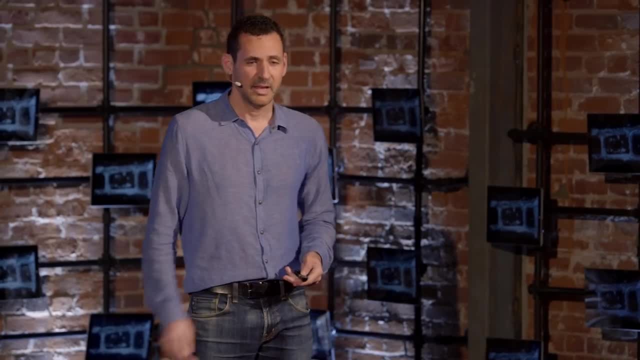 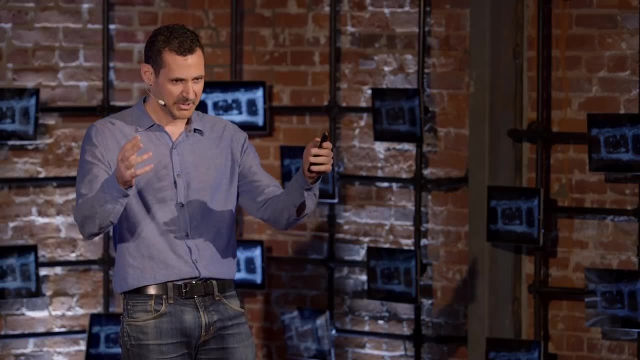 Don't worry, Mom, it's just a theory, And that is ordinarily when you're looking at something or someone, or a face, for instance, you don't consciously perceive every last detail all at once, every pore, every eyelash. Your brain is constantly simplifying and filtering what you're looking at to make it more comprehensible. But people who've had psychedelic experiences sometimes say that it feels as if those filters are removed and all of the information gets through at once and it's sort of sensory overload. 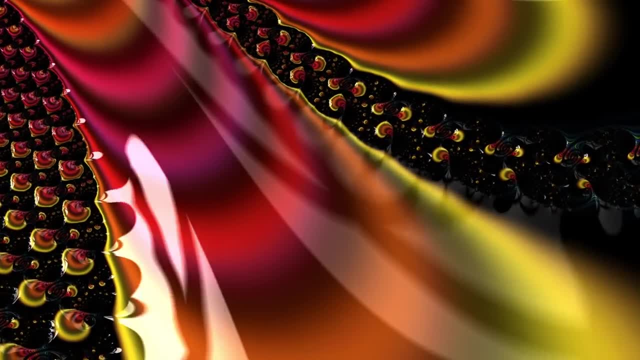 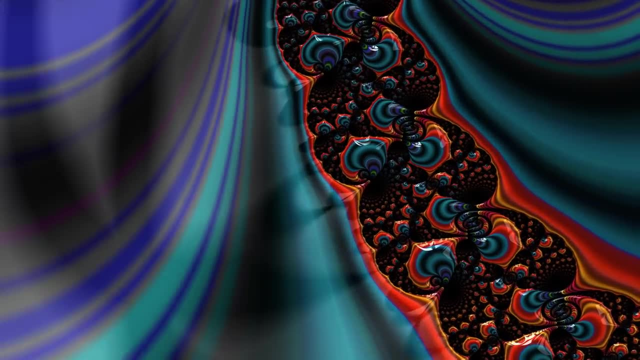 And I suspect that when you're looking at fractals like this, that the reason it has a similar effect is that they're so complicated. your brain doesn't know how to simplify them, And so the filters don't work and all the information gets straight through. 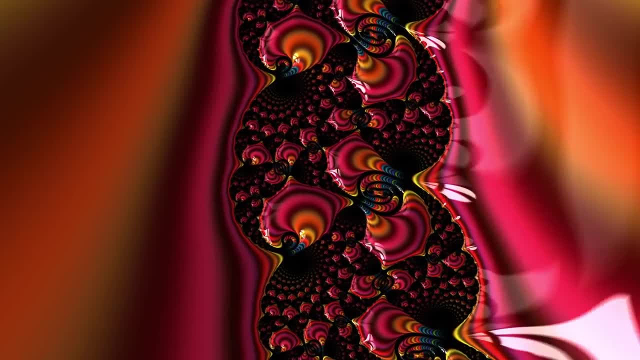 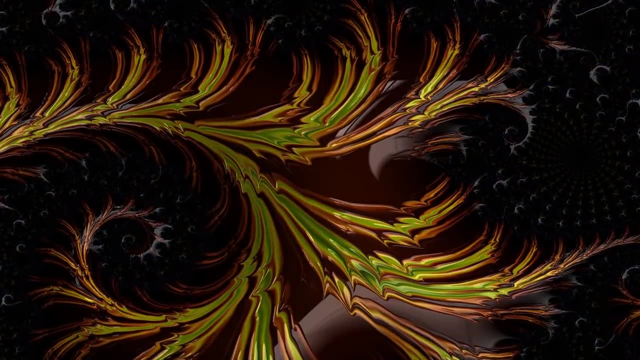 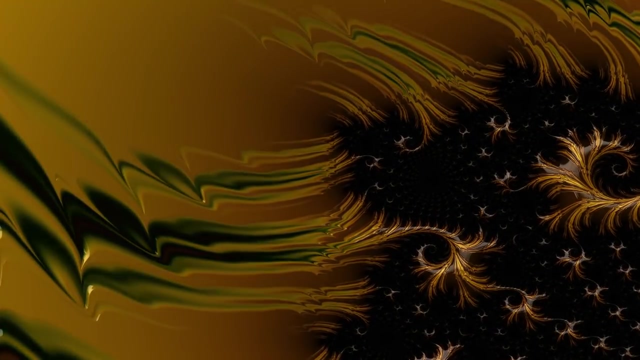 and it creates an overwhelming sensory experience. And there are some interesting implications of this, Because recently there have been some preliminary studies that seem to show that controlled doses of chemicals like psilocybin can actually have a very measurable positive effect for some patients suffering from PTSD or depression. 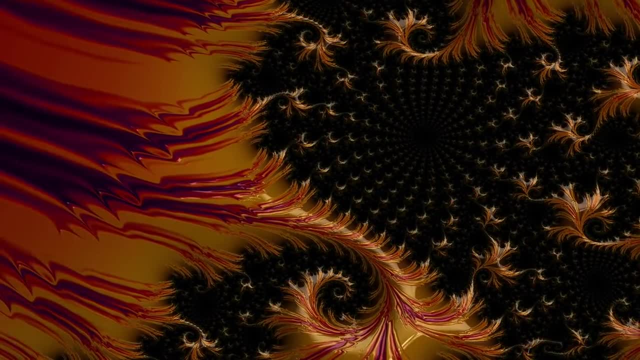 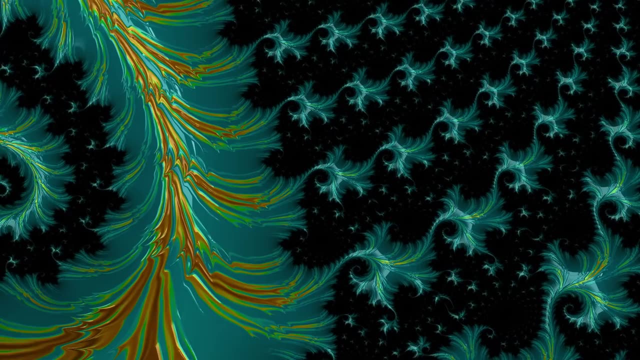 And if these fractal images are activating some of the same areas of the brain, it's possible they might have some of the same beneficial effects. And although it's anecdotal, some of the feedback that we've received seems to bear this out. 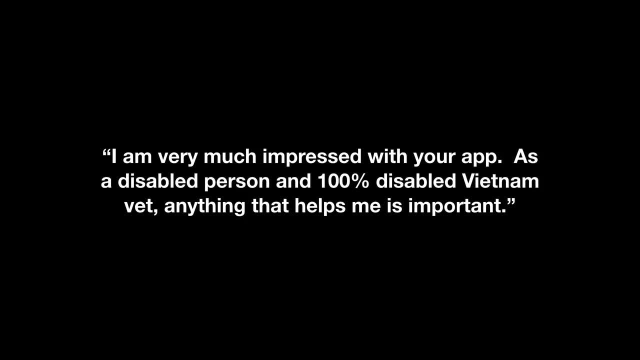 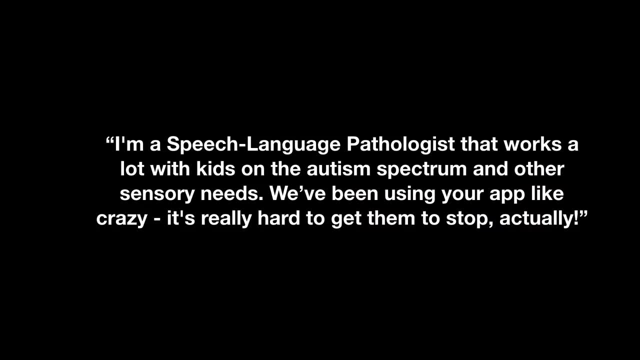 I am very much impressed with your app. As a disabled person and a 100% disabled Vietnam vet, anything that helps me is important. I'm a speech-language pathologist that works a lot with kids on the autism spectrum and other sensory needs. 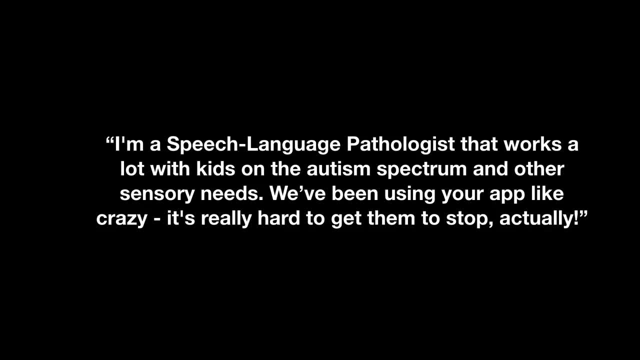 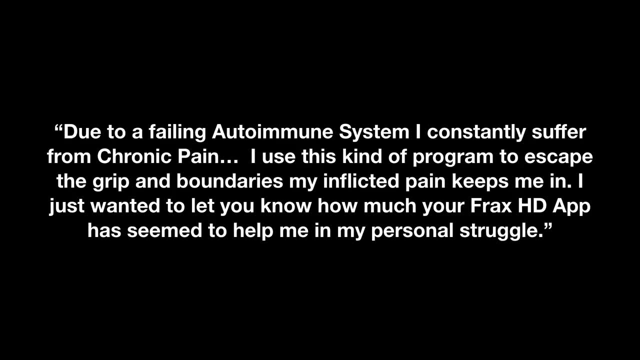 We've been using your app like crazy. It's really hard to get them to stop. actually, Due to a failing autoimmune system, I constantly suffer from chronic pain. I use this kind of program to escape the grip and boundaries my inflicted pain keeps me in. 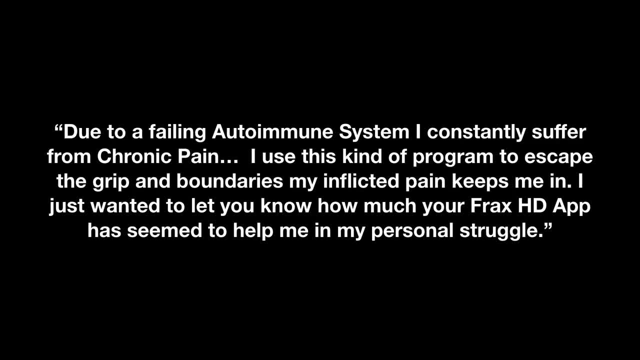 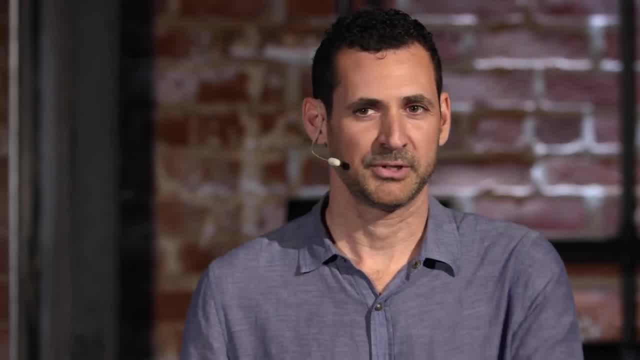 I just wanted to let you know how much your app has seemed to help me in my personal struggle. And so, if fractals can affect the brain to this extent, that leads to another interesting question, Because we know that the lungs are a fractal. 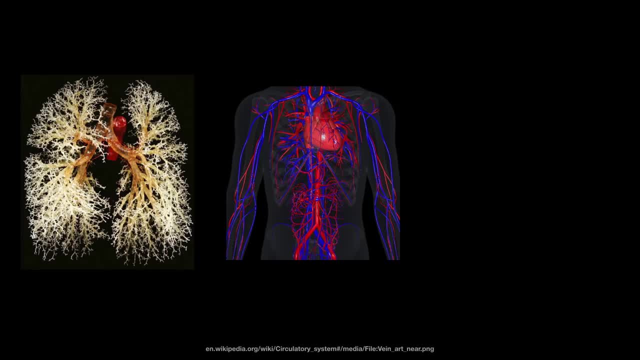 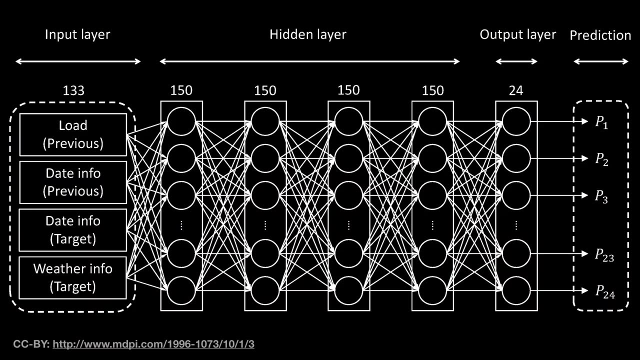 and the circulatory system is a fractal. could the brain be a fractal as well? One way to think about this question is through the lens of artificial intelligence and machine learning, the tools that we have to model and simulate what's going on inside the brain. 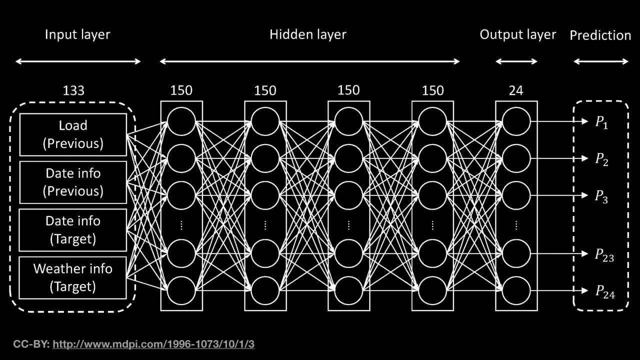 And some of the most successful of these deep neural networks operate on a principle where they're processing information over and over again, while periodically feeding back in the original information to keep the process going. And that might sound a little bit familiar, because it actually is quite similar. 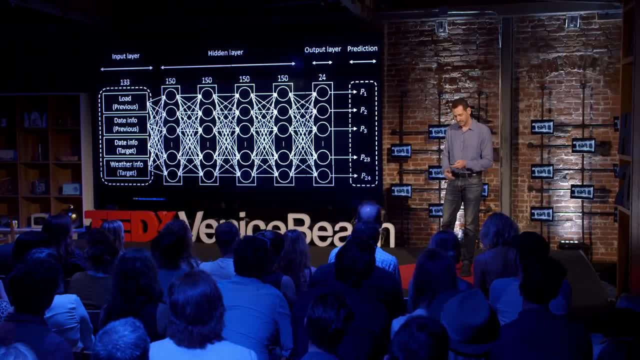 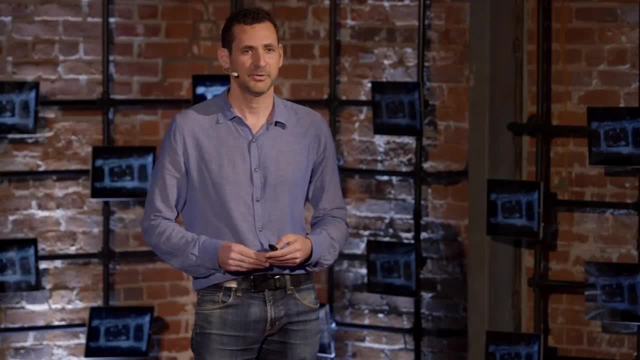 to the way that Mandelbrot's fractal equation works, And what that suggests is that, whether or not the brain is a fractal, it's something much more powerful. It's an engine for generating fractal levels of complexity. So it could be that the brain is not a fractal.